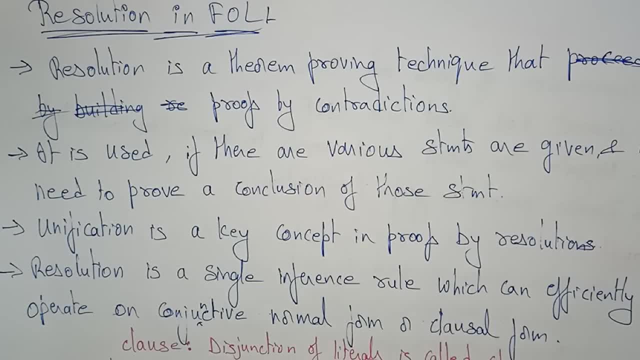 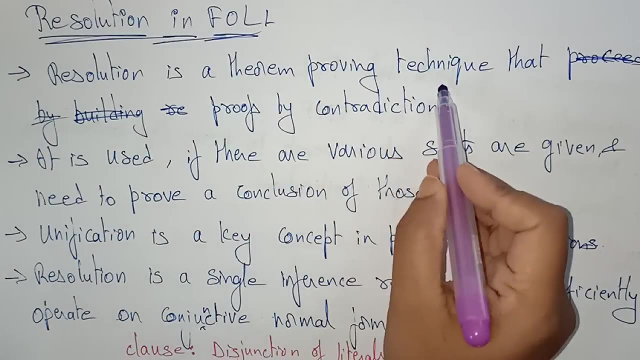 Hi students, welcome back. Let's continue with the subject: artificial intelligence. The next topic in the subject is a resolution in first order logic. Okay, now let's see what is the resolution. in first order logic, A resolution is a theorem proving technique that proves by: 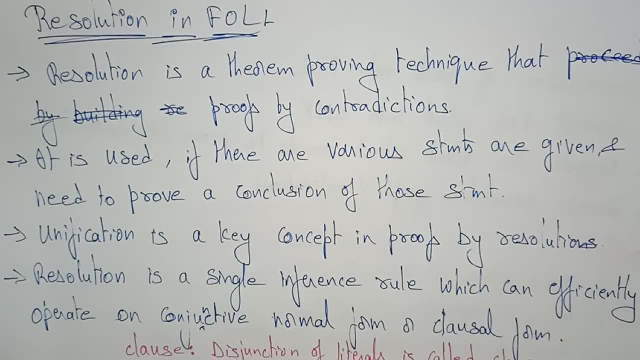 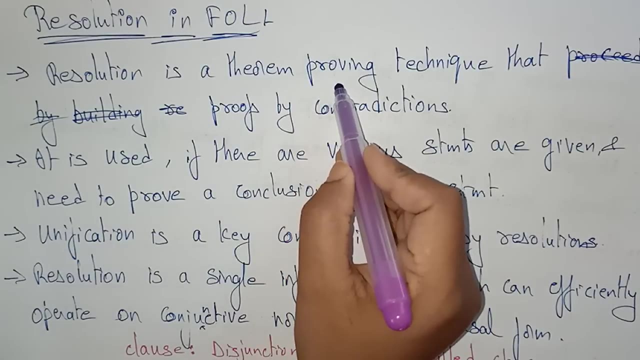 contradiction. The first thing that you have to remember that if you want to solve a resolution problem, you have to prove contradiction. Whenever the contradiction is success, then the solution is resolute. Okay, so a resolution theorem is a proving technique. theorem proving technique that proves by contradiction. It is used if there are various. 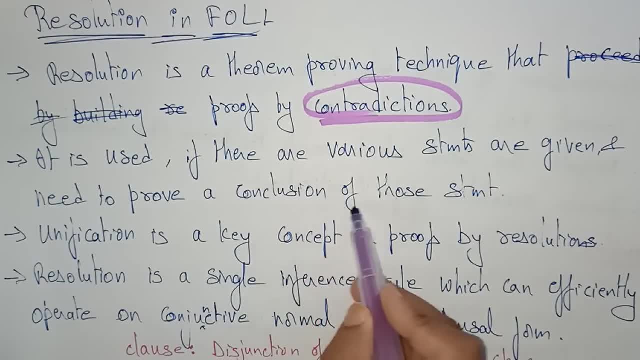 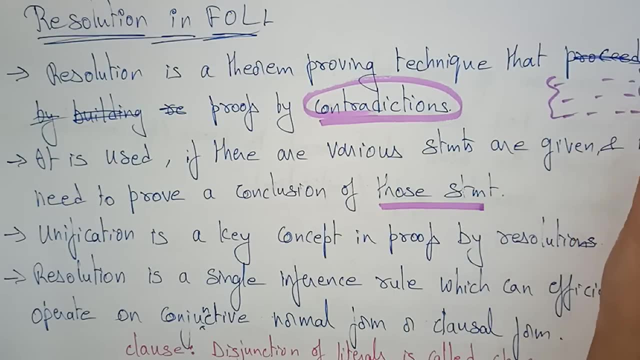 statements are given and we need to prove a conclusion of those statements. Let's take: there are so many statements in the problem. Okay, so with the help of those statements, we need to prove a conclusion of those statements. So let's take: there are so many statements in the 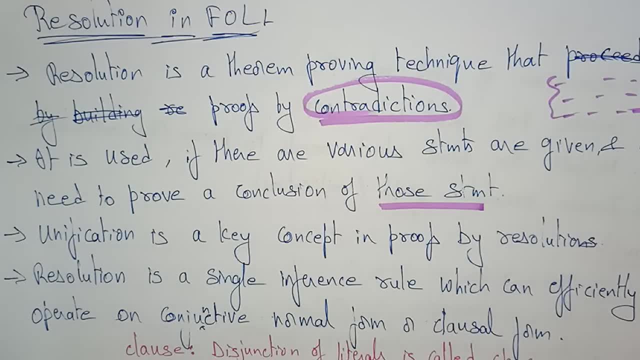 problem. Okay, so we have to prove, we have to get a conclusion. Okay, so some different questions will be arised. So by seeing the different questions and you will get different answers In the different answers, you need to get one conclusion in that. So in that cases we will. 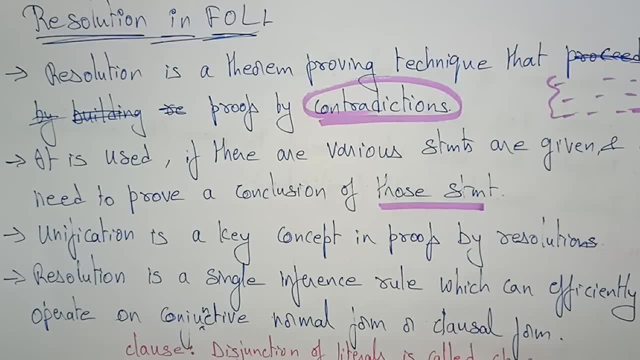 use this resolution concept in the artificial intelligence. Okay, so the resolution is used if there are various statements are given and we need to prove a conclusion of those statements, And unification is a theorem proving technique that proves by contradiction. So let's take 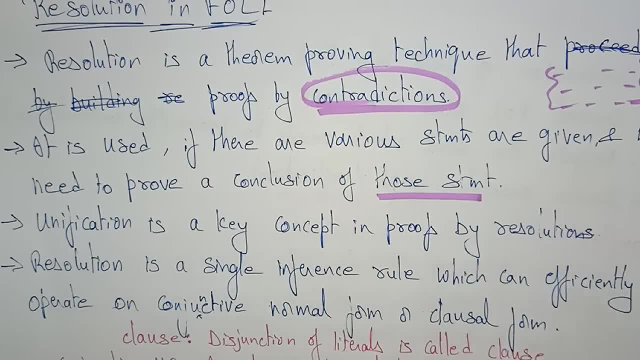 that. So let's first take the unification concept in the universal unit equation, And there are three different types of unification tasks in the artificial intelligence. One is the probability, the approaches back, and this the local theory as well as the human theory. 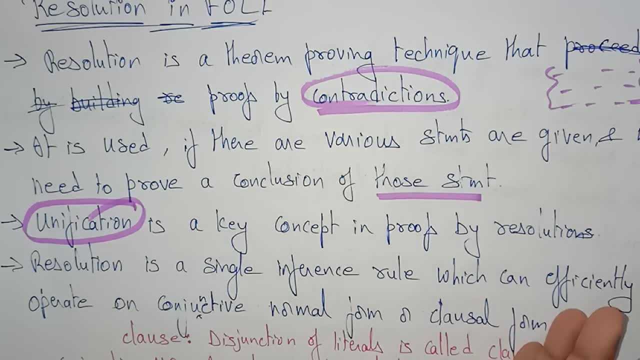 When we talk about this, let's say we want to rule out this Trading Table. So here we need to calculate these bones by sells. So there are only a number of reasons If it's a probability of the process by 보면 ofropалось and de Ramsày, and then there can be other. reasons by theйmovement popular health of the". You played the part. So, basically, this is what does the procedure? Okay, and then youте pose on the father's new activity that you played with me- who have to attend a celebration. Let's see how you can figure this out. You might ask me the scooter and 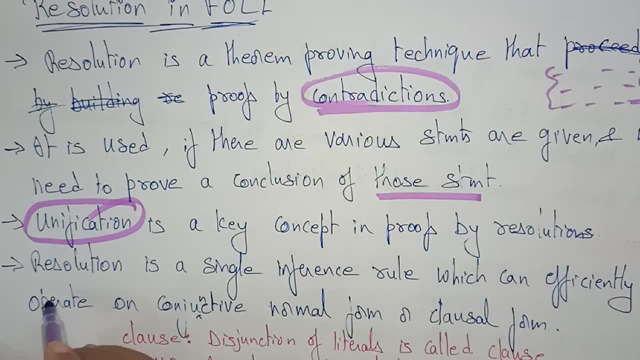 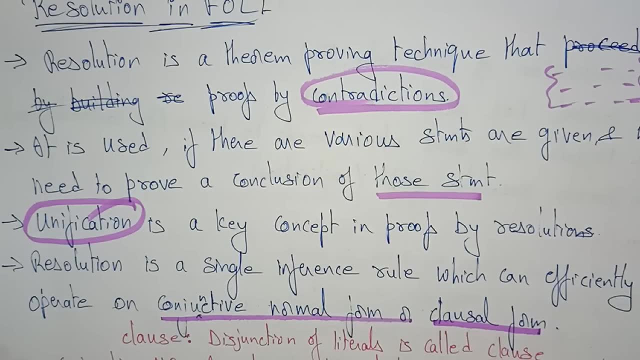 So first for that is some nons park channel problems. what is this resolution? topic is resolution is a single into inference rules which can efficiently operate on conjunctive normal forms or clause forms. okay, so here we are: resolution can be solved and it can efficiently. 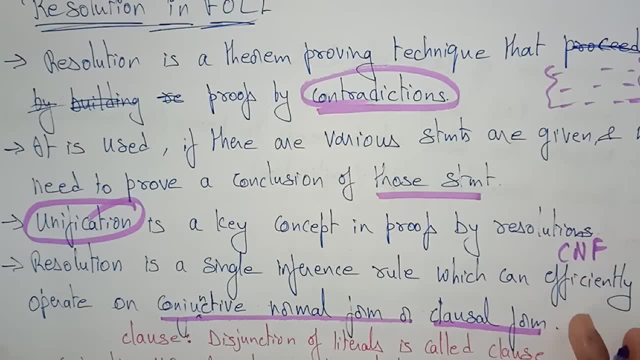 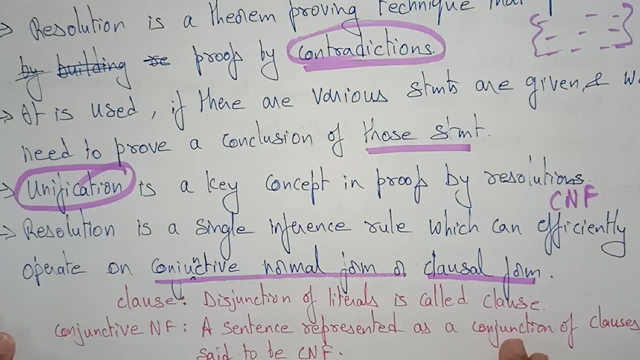 operated on CNF, that is a conjunctive normal forms. so clauses is the distinction of literals is called clause, whereas conjunctive normal form is a sentence represented as a conjunction of clauses is said to be CNF. so first thing is: whatever the first order logic is there, that first order logic has to. 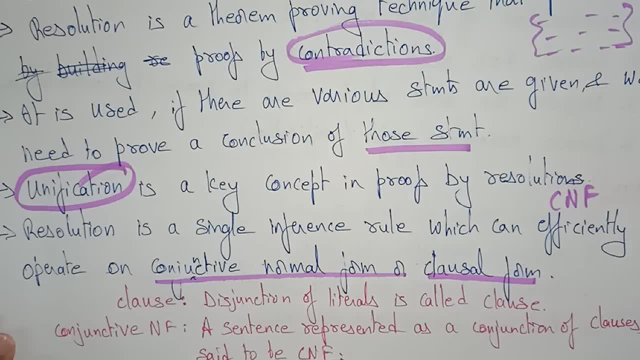 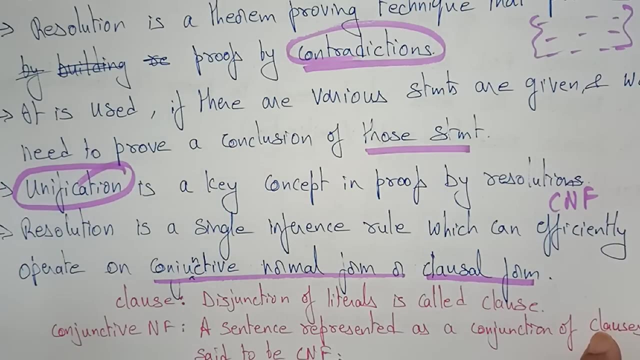 be converted into these conjunction normal form, then only you can prove by resolution. means, with the help of the conduct to normal form statements. you can prove by resolution, whatever the statements they are given. means we can find the various statements that are given and then we can provide you with a single conjunction of clause. is there? 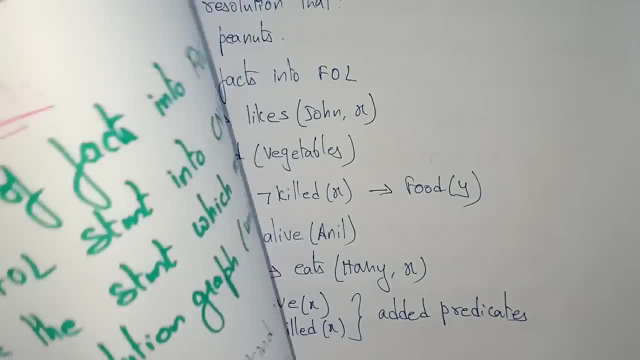 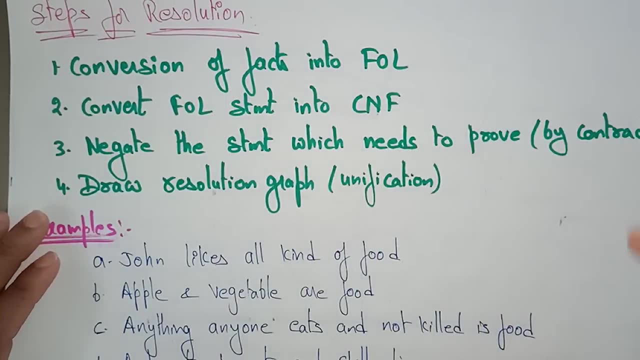 And we need to prove a conclusion of those statements. So now let's see the steps for resolution. These are the important. So based on these steps, we are going to solve the problem one by one. So first is conversion of facts into first order logic. 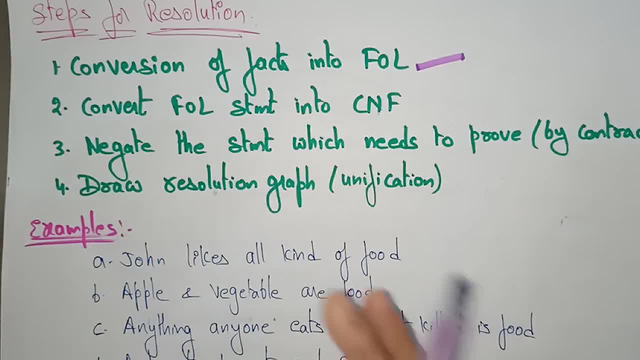 Whatever the statements, the series of statements they are, given, that statement has to be first converted into first order logic. You know, the first order logic, The first order logic consisting of the facts, and it will be used as some connectivities. Okay, so I already explained about the first order logic. 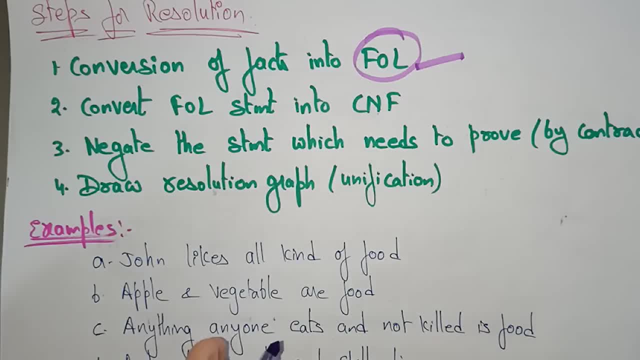 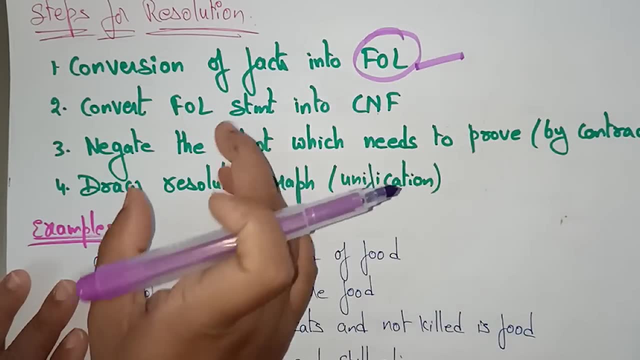 It has the statements like objects, connectivities, functions, relationships, Everything will be there, the statement. So after converting the first order logic that statements again, you have to convert it into CNF. First, convert the facts into first order logic. 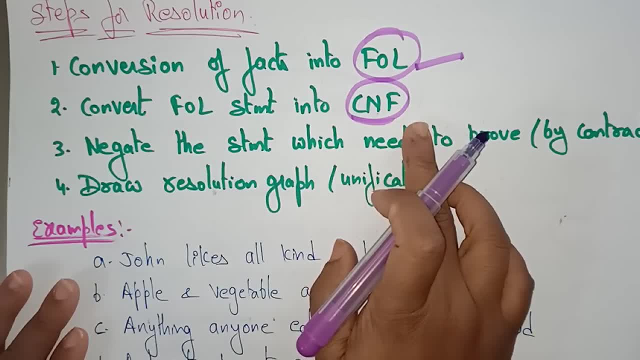 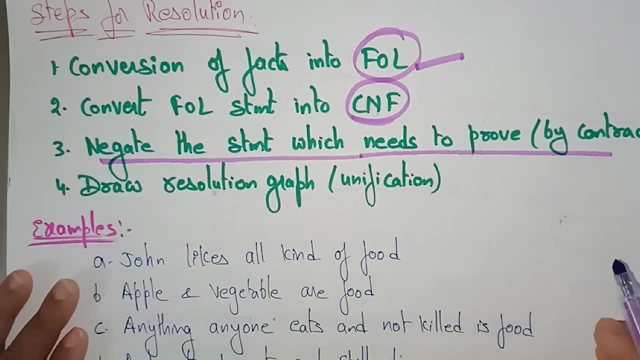 Next, convert the first order logic into conjunctive normal forms. After, whatever the conjunctive normal you are getting, negate the statement which needed to be proved by contradiction. So you have to negate the statement. Whatever the statement you are thinking, that has to be proved. 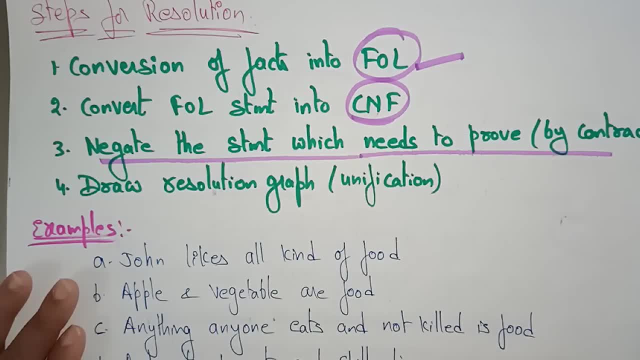 Just take that statement, negate. Okay, you just take the contradiction of that statement and draw the resolution graph. So these are the four steps for the resolution. What are this? first, convert the given facts into first order logic. After that, the first order logic is converted into CNF. 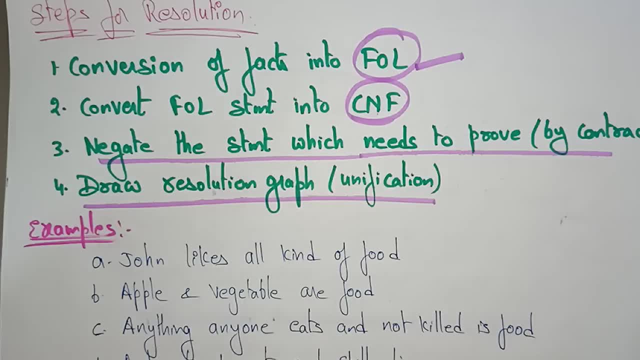 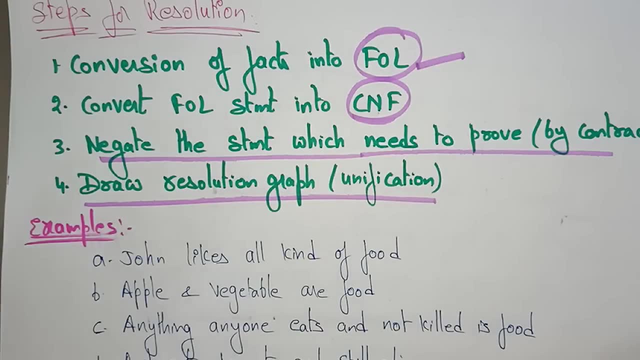 Okay, conjunctive, normal forms. After that you have to, whatever the statement that you get, that statement you need to be negate and you have to prove that by contradiction. And we have to draw the resolution graph with the help of unification means, by substitution method. 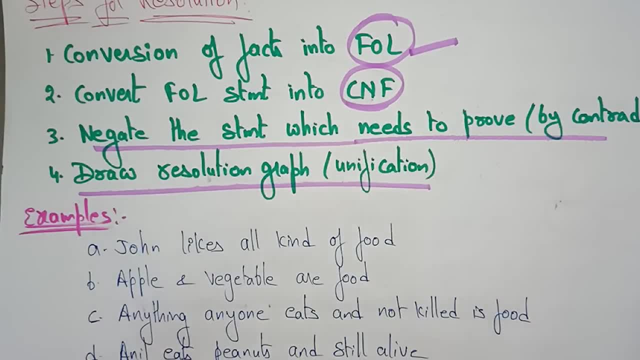 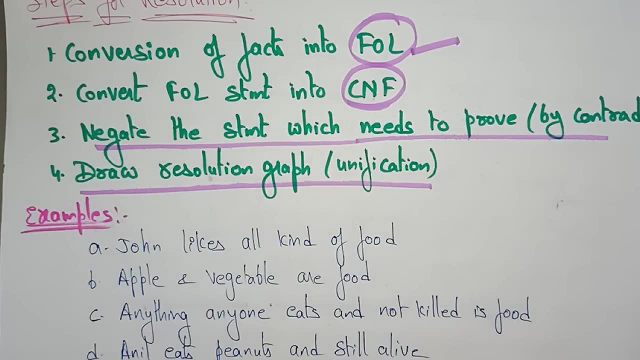 So let's see some example. So here in this video I'll explain with some example. Suppose. if you didn't understand these examples, don't worry, And I'll explain one more example in the next video with simple concept. Okay, here I am taking a big problem. 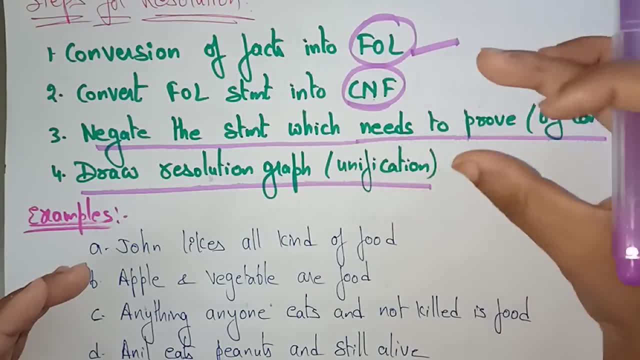 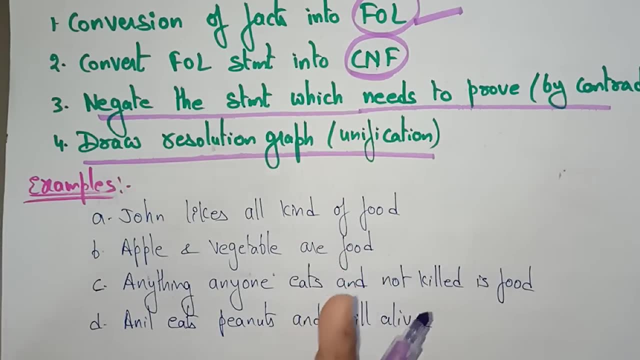 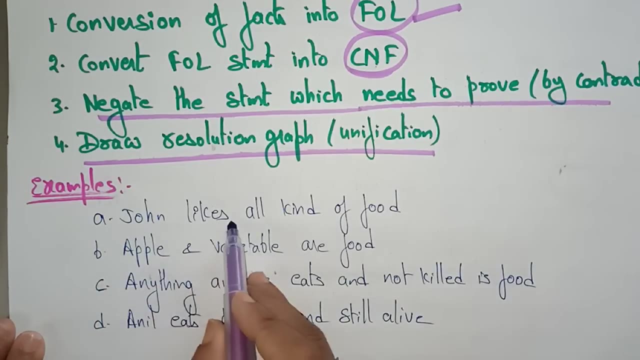 By applying these rules, these steps, to solve the resolution. So here the example is. I'm having a series of steps in their statements. I need to find the conclusion by using the resolution. Okay, so here the steps. or John likes all kind of food. 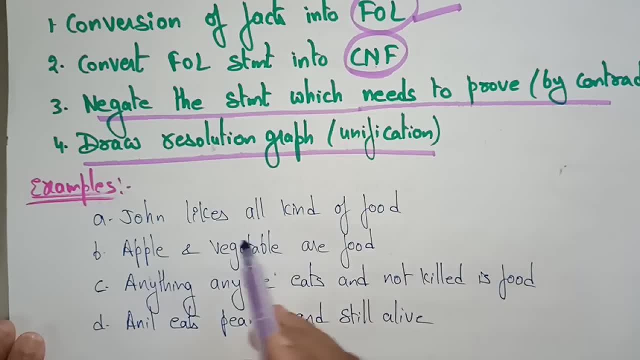 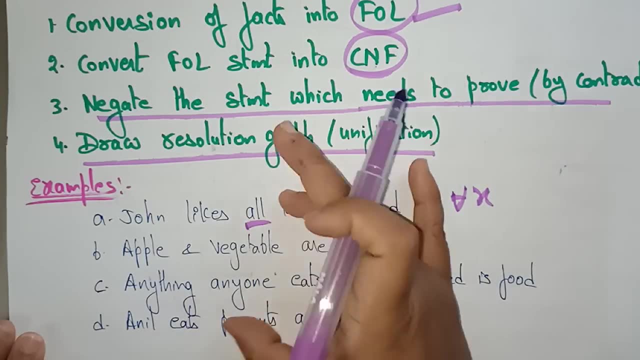 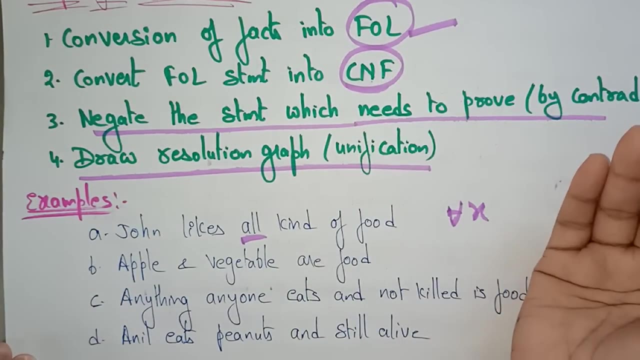 Okay, John is a person. He likes all kind of food, So whenever you see this, it is nothing, but you have to use the universal quantifiers. Okay, so means You have to convert these statements into FOL. FOL is consisting of the quantifiers: the universal and existential quantifiers. 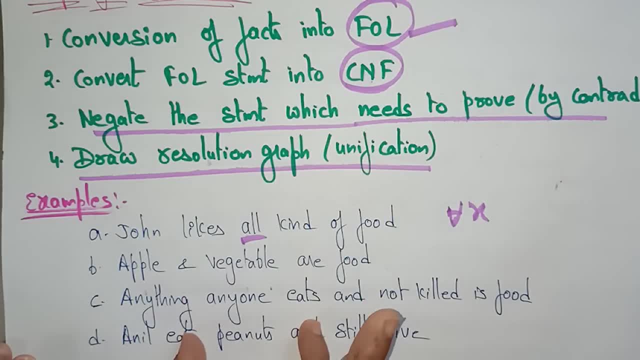 With the help of those quantifiers you have to represent the statements. So these are all the facts. John likes all kind of food. Apple and vegetables are food. Anything anyone eats and not kill, it is food. Anil eats peanut and still alive. 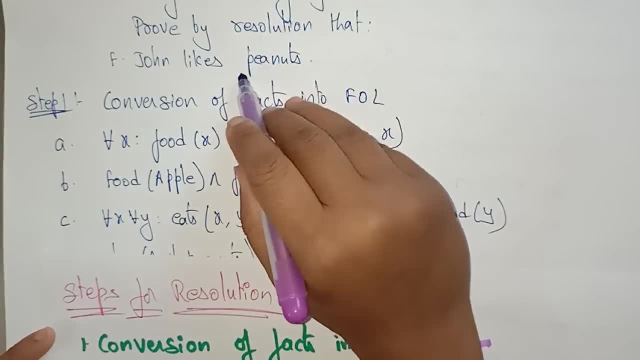 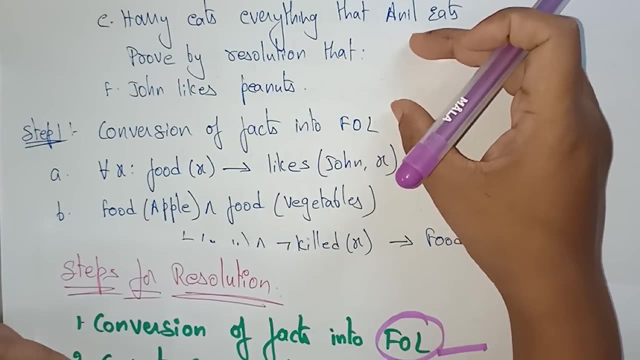 And Harry eats everything that Anil eats, and prove by resolution that John likes peanut. So these are the steps, whatever the statements they are given, So we have to prove John likes peanut. So in the third step, what I had to take, 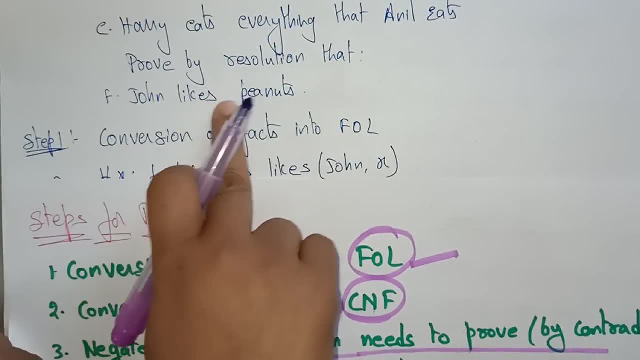 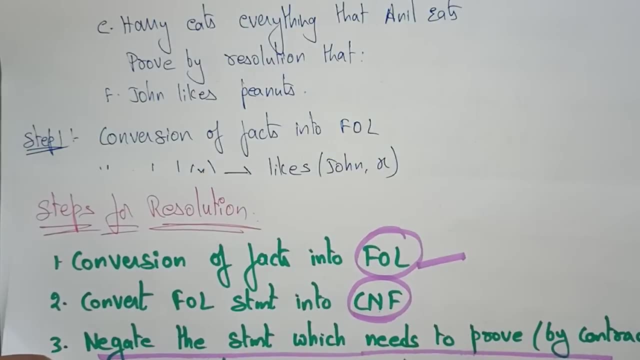 I have to take the negate, the statement which need to be proven. John does not like the peanut. I have to take to prove that condition. But first, whatever the steps they are given, convert these steps into first order logic. How So? first statement is: John likes all kind of food. 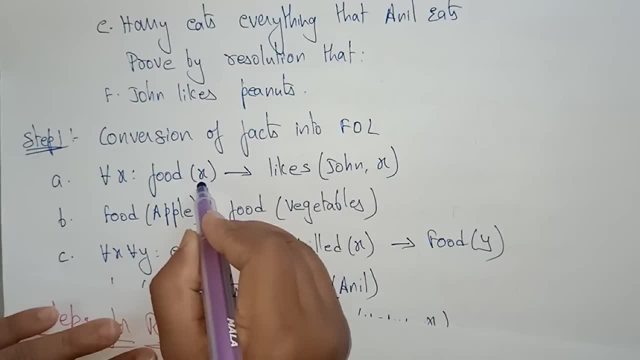 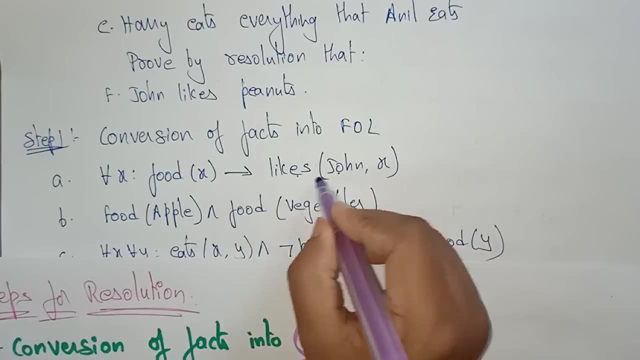 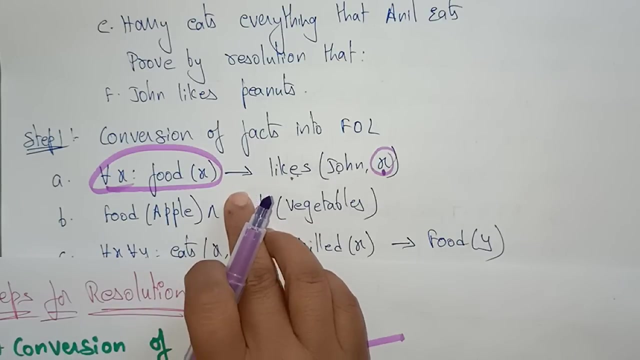 That means let's take for all eggs The food X likes, that is, you have to represent these statements. John likes all kind of food. John likes food That is all kind of food, For all eggs food. So universal quantifier is represented with the implies. 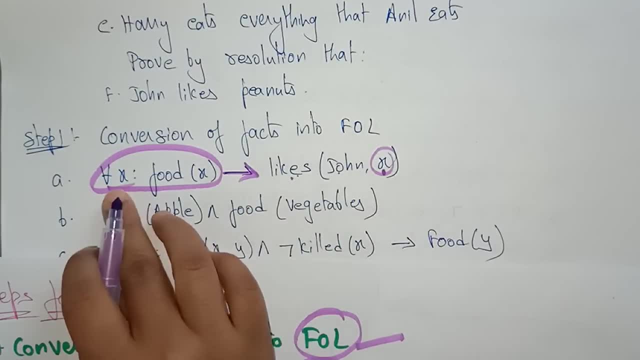 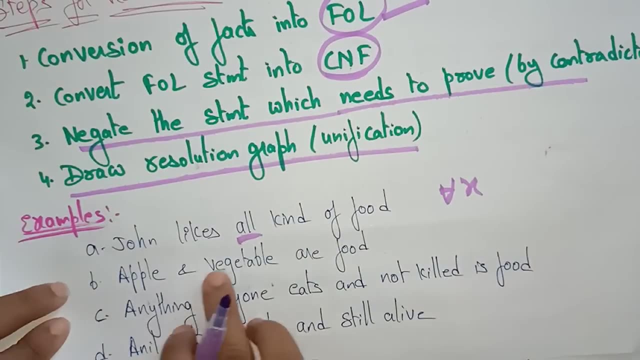 It can be work on implies. So for all eggs food of X. John likes that food. So the first statement is over. The second statement: Apple and vegetables are food Means. here, apple is a food and vegetable is also a food. 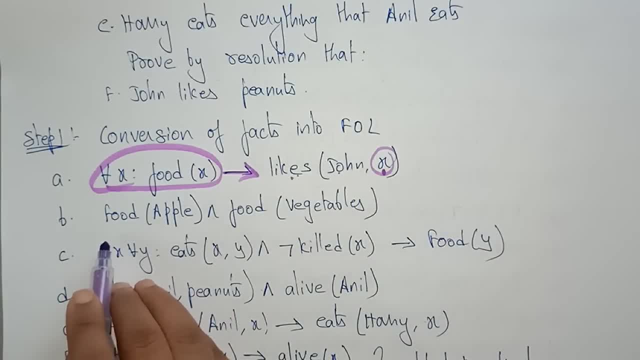 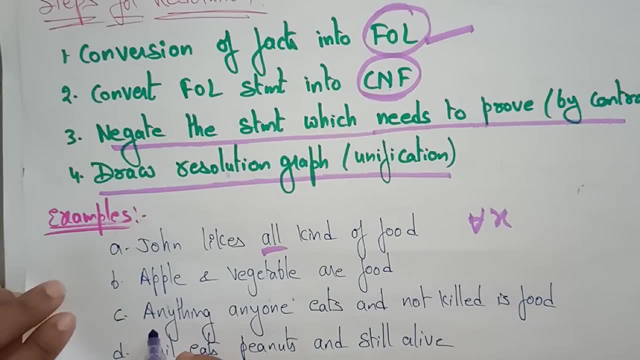 So that you can represent it as in the first order logic: food, Apple is a food and vegetable is a food. Okay, second statement is over Now. third statement: I have to represent it in first order logic. Anything anyone eats and not killed is food. 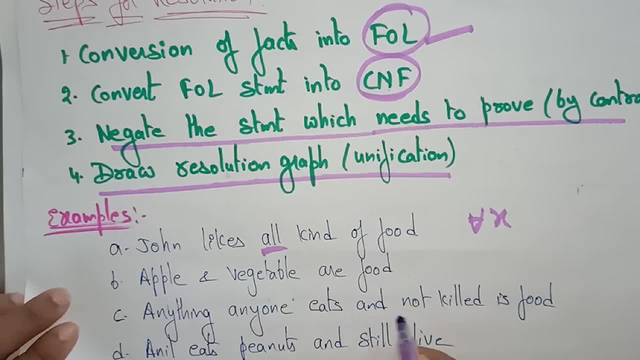 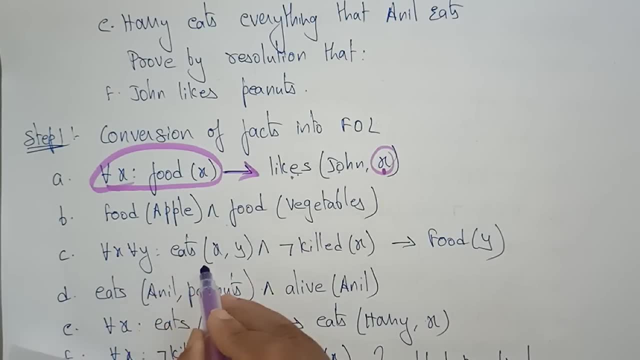 Anything anyone eats and not killed is food. So that is here, Here, that for all X, for all Y, eats X, Y and not killed, X. That is the food is not food, is it's not killed. yet They are saying that not killed is food. 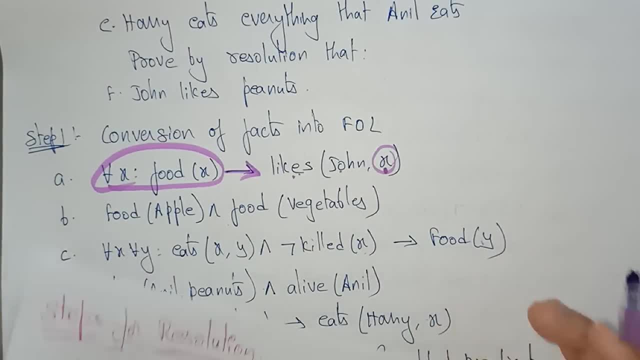 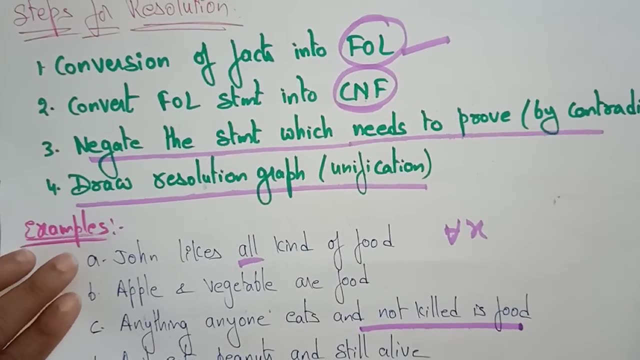 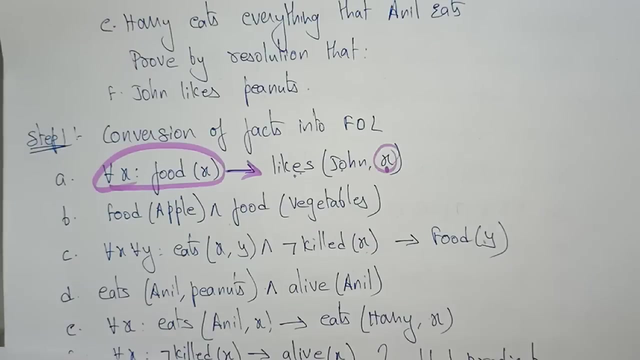 So not killed implies food of Y. So this, this statement, I have represented in the first order logic. Next one: I need eats peanuts and still alive. So this is a fourth statement I have to convert into first order logic: Anil eats peanuts and still alive. 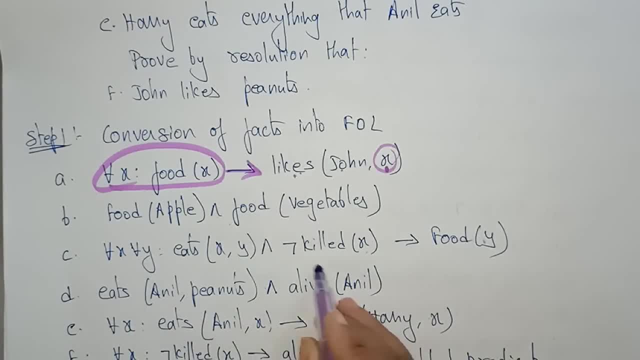 So Anil eats peanut and he is still alive. It's peanut and he is still alive. Okay, next statement: Harry eats everything that Anil eats. So Harry eats everything that Anil eats. So see here for all X. Okay, 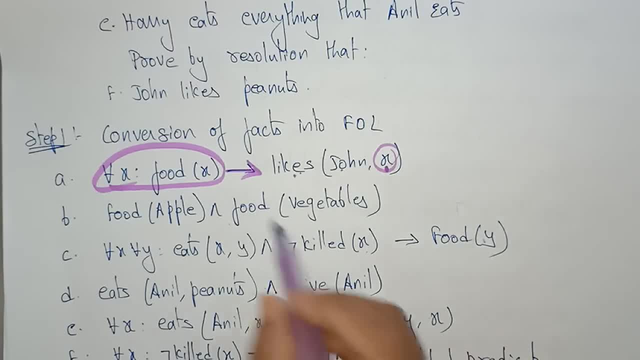 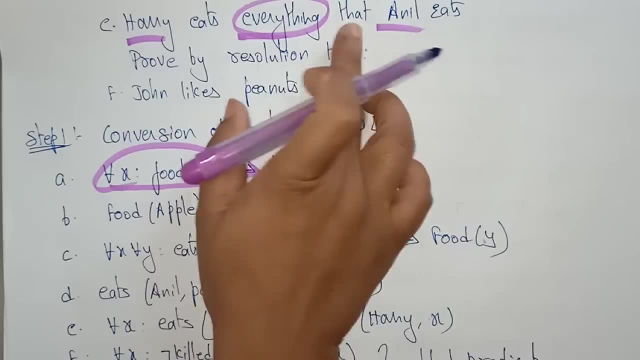 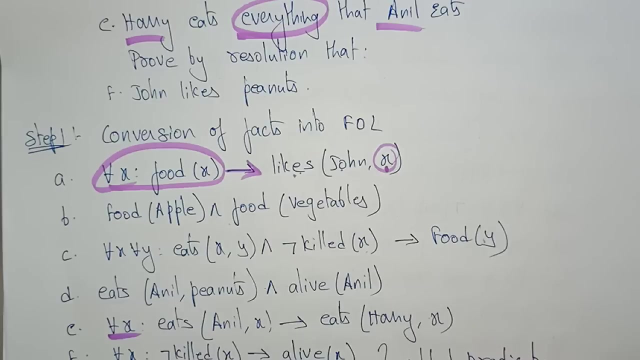 Anil eats X and Harry also eats that X, because Harry eats everything that Anil eats. So Harry and Anil both will eat the same, Whatever. the Harry eats everything that Anil also eats. So that's why Anil eats X means the Harry also eats X, for all X. 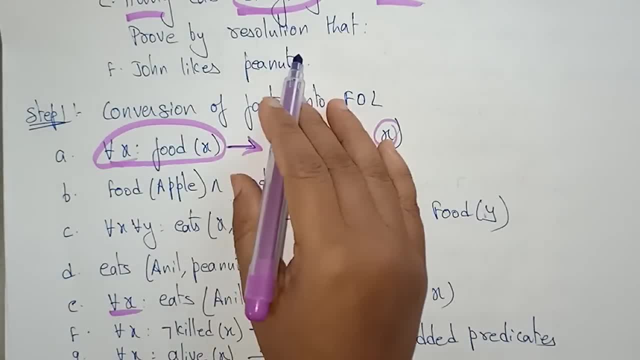 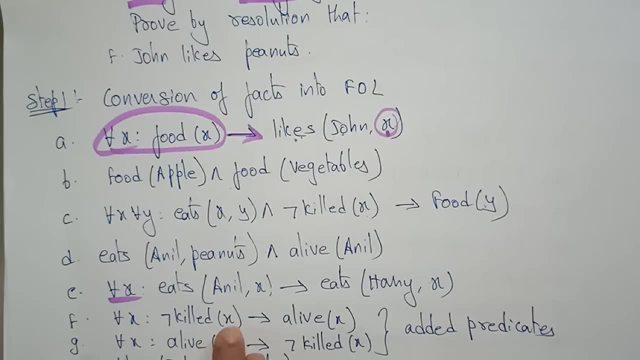 Okay, is it clear? So I had taken that. I had to prove by resolution that John likes peanuts, So further I had to take some added predicates here. That is, if suppose not killed means obviously it is alive. So alive means not killed. 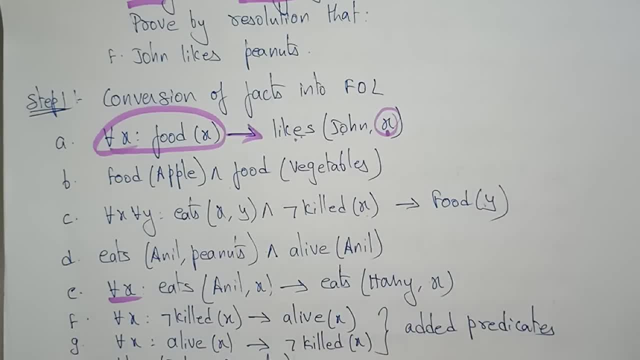 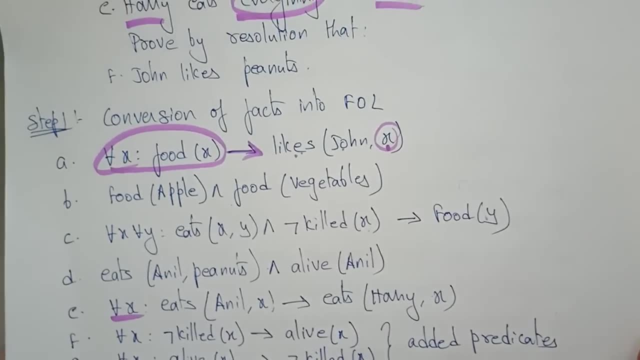 So both are the same. I had taken the added. this predicates next: John likes peanut, John likes peanut. So I represented in the predicate form. So this is a step one, Now coming to the step two. So what is the step two? 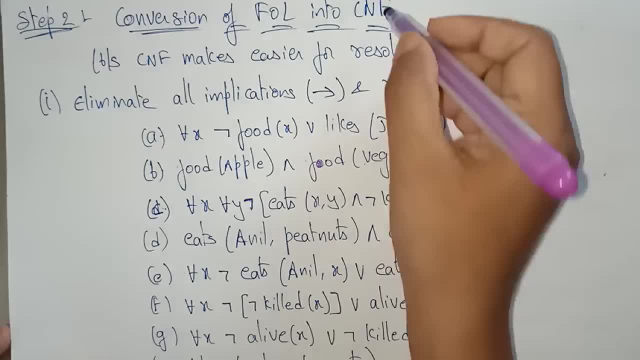 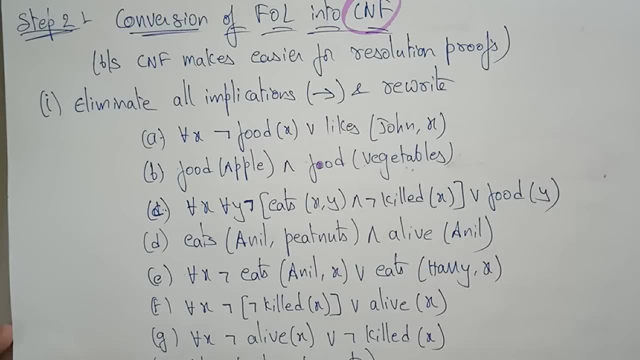 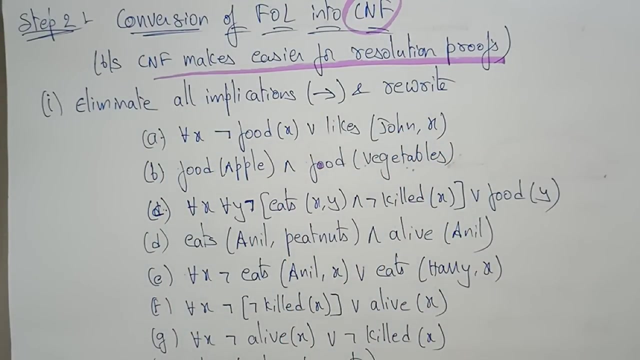 Whatever the first order logic that I converted, that I have to convert it into conjunctive normal form, CNF. That is a step two Why I'm converting into CNF: because CNF makes easier for resolution proofs. So for that sake we are converting the FOL into CNF. 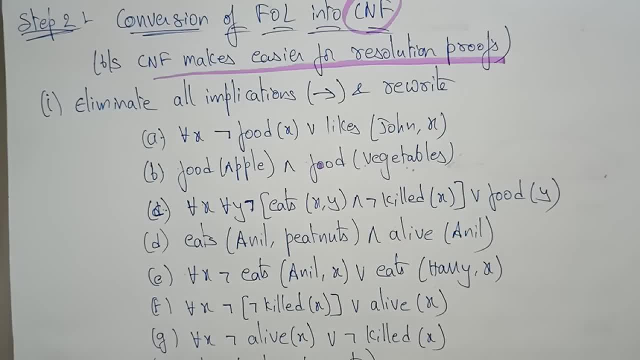 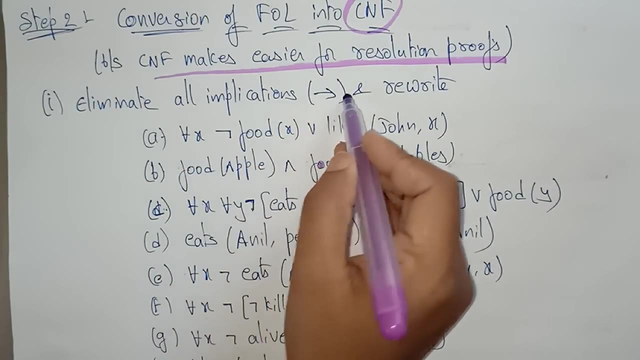 So how you're going to convert the given FOL into CNF. There are series of steps we have to be followed. There are total five steps here, Six steps that need to how it is going to be converted into CNF. The first thing is eliminate all implications. 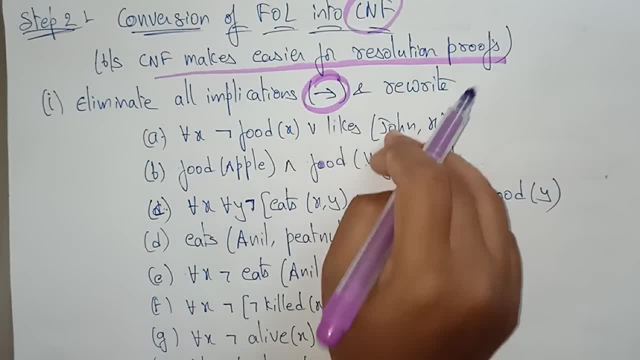 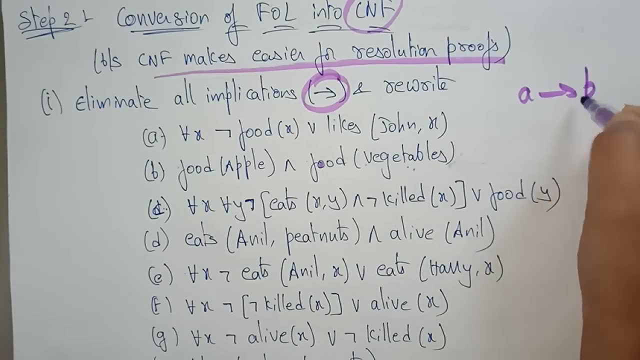 So wherever the implication symbol is there that you have to eliminate and rewrite, Then you'll get it out how I can rewrite the implication. Suppose A implies B is there, so I can eliminate these A implies B by writing Nagate A or B. So this: both are the same. 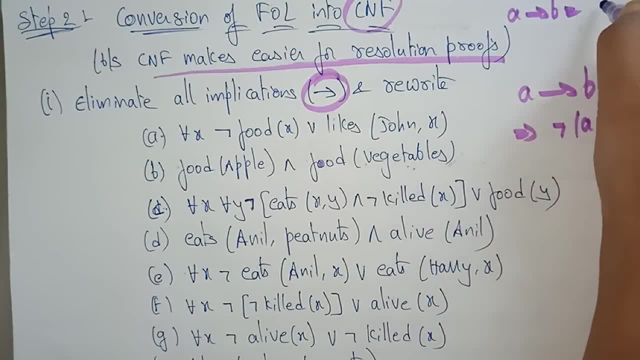 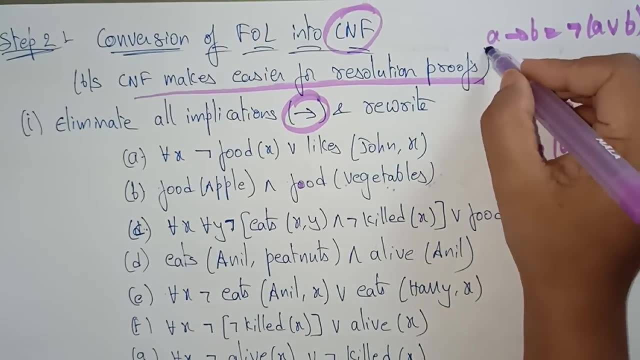 Okay, that means A imply B is equal to Nagate A or B. So here the implication is eliminated or not? Okay, So this is a formula, If you want to. wherever the imply symbol is there, These imply symbol, It has to be eliminated by rewriting it as Nagate A or B. 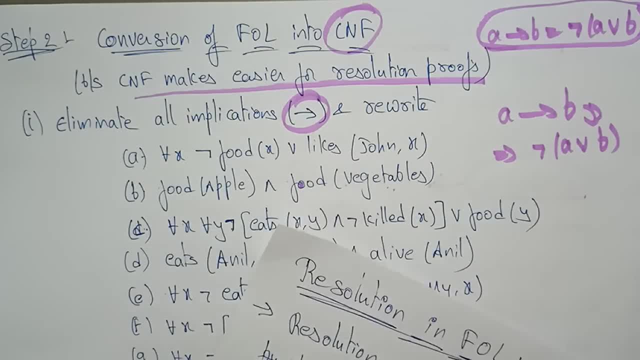 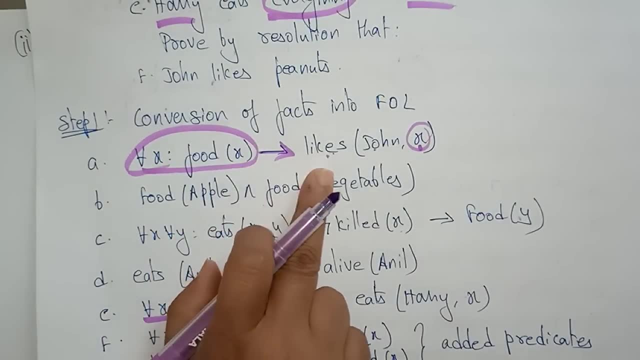 So let's see wherever the negation imply symbol is there that I need to be eliminated. So the first in the first, what is this? food of X implies likes John of X. So I want to eliminate this. This is: let's take: this is A and this is B. A implies B. 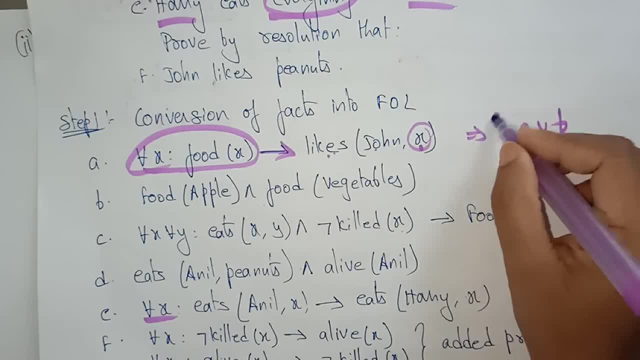 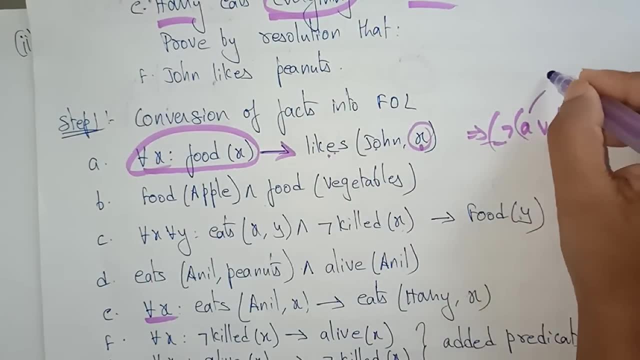 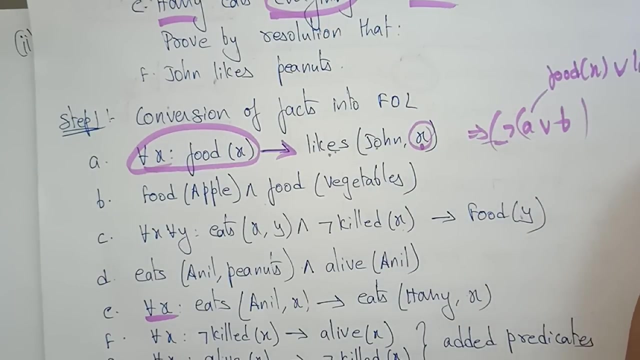 So I have to write it as Nagate A or B. Okay, I have to write this as Nagate A or B. So how I can write So here: A is food of X, So in place of A, write food of X. or in place of B write likes John, comma X, like that. 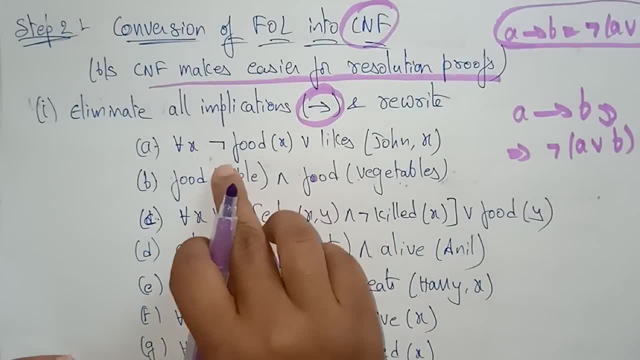 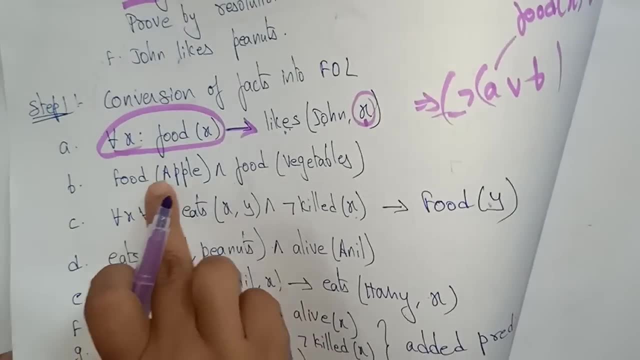 Okay, put negation here. So I just put negation here. Negation food of X or likes John, comma X, So in the same way. So in the second step there is no implies, There is no imply, So write as it is in the third step. 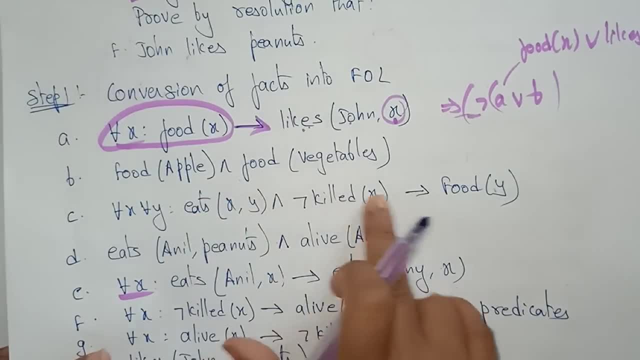 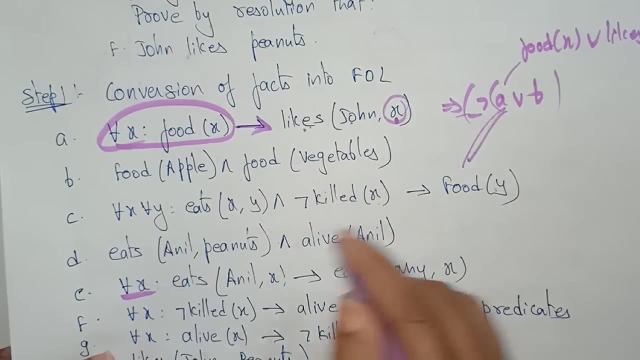 There is an implies, There is an implies. Let's take this is A and implies B. A implies B. Apply the formula Nagate A or B, So you have to represent these statement in the form like this: Nagate A or B. 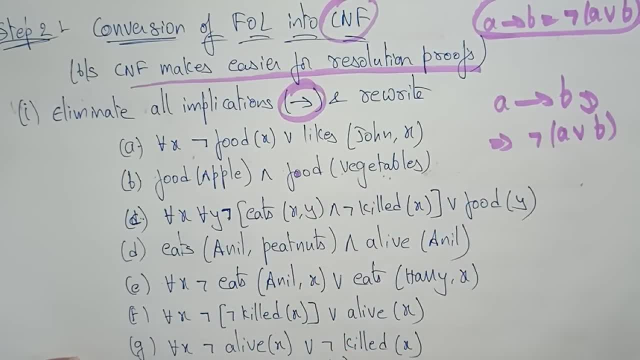 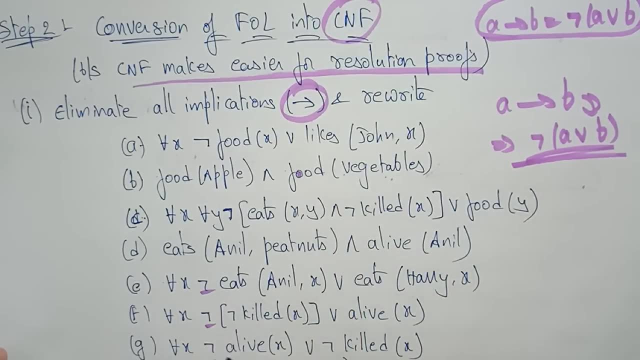 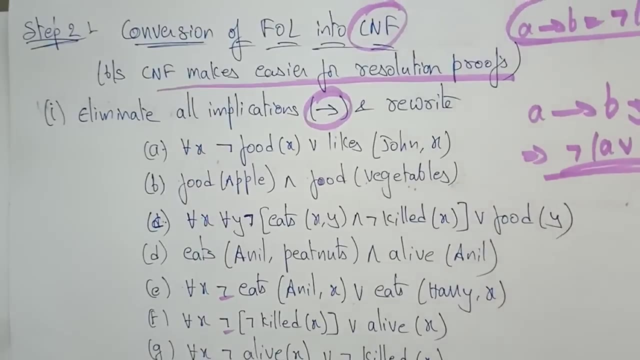 So, whatever the statements I have written, just eliminate all implications and write in this form: So then here: observe: there is no implication here, Only the negations will be there. So I eliminated the imply symbols and rewrite with this formula. There's a first step. 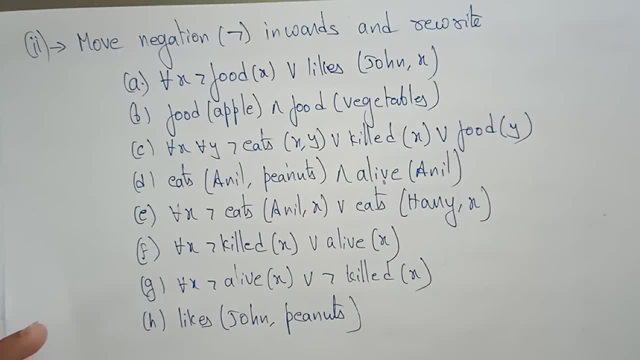 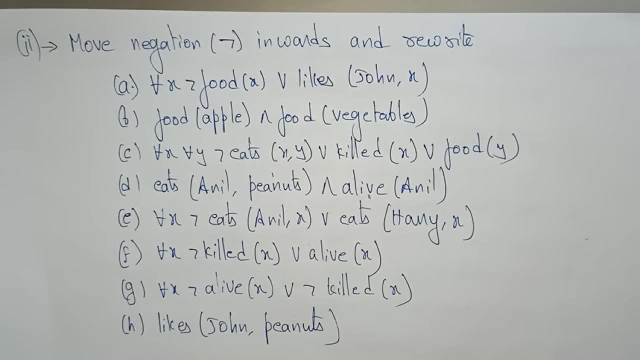 In the second step. that is the first thing. And the second thing, to convert the first order logic into conjunctive normal form is move the negation inwards and rewrite. So whatever the negation that is there. So here I apply, I move, 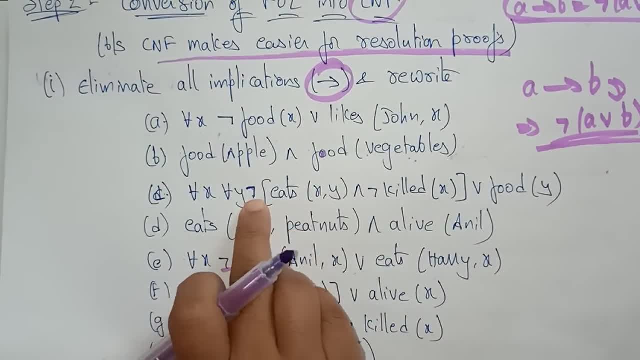 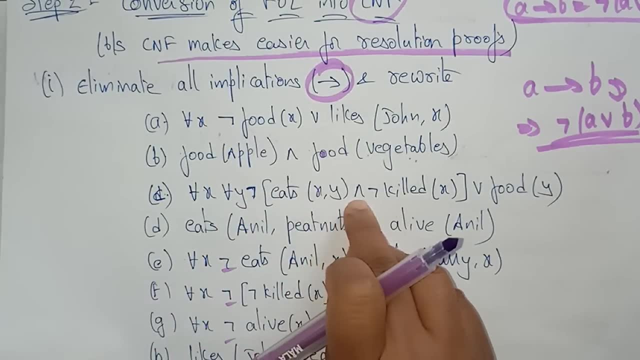 I have to move that negation inwards. That means so here suppose negation is there, Here the brackets is there. I want to move that negation into inside Nagate eats X, comma Y, and here end becomes OR. Whenever the negate application is there, end becomes OR. 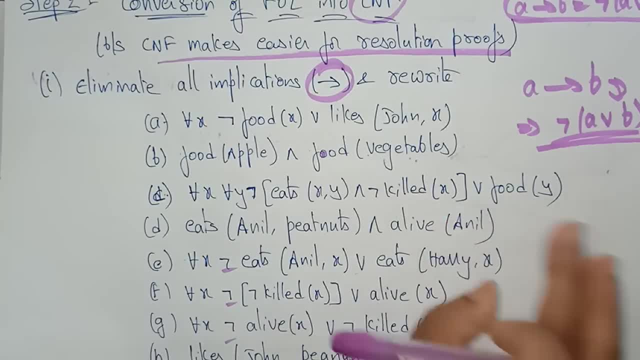 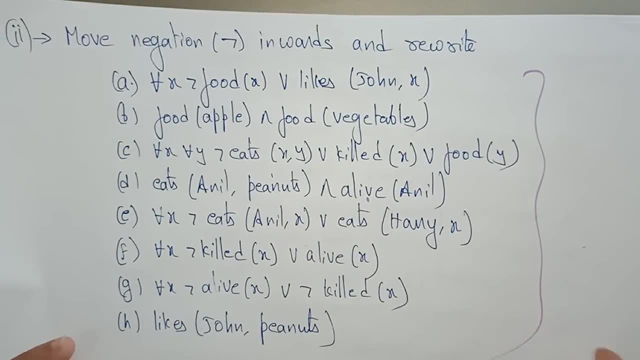 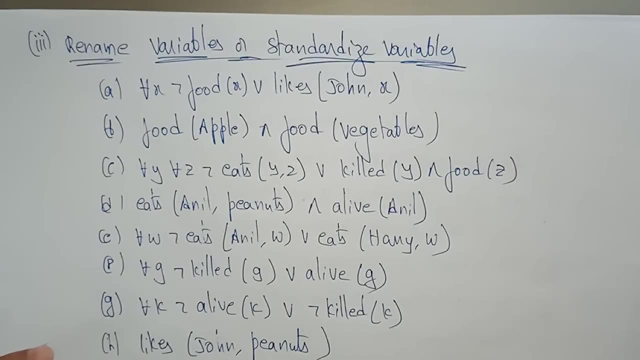 And this negate, negate will be cancel and it becomes killed X, like that. OK, So that is the second step: more negation, inverse and rewrite. So I rewrite all the statement by moving the negation inwards. Next third step: in the third, after that, I have eliminated the implications. 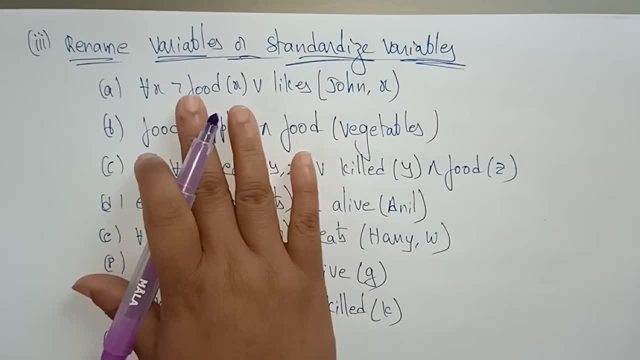 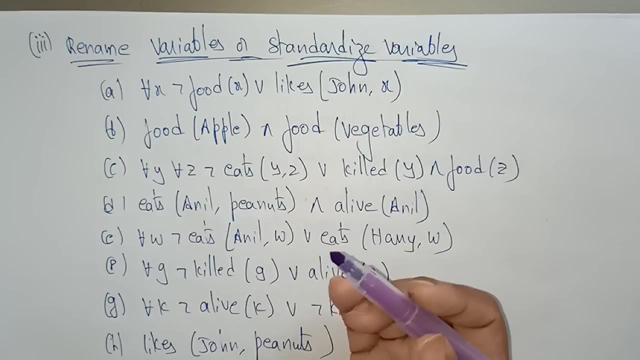 I have inverse the negation. Now rename the variables or standardization variables. So to make somewhat difference without confusion, you just rename the variables. So wherever the X, Y is there, just rename all the variables with Y, Z, Z, K, whatever it may be. 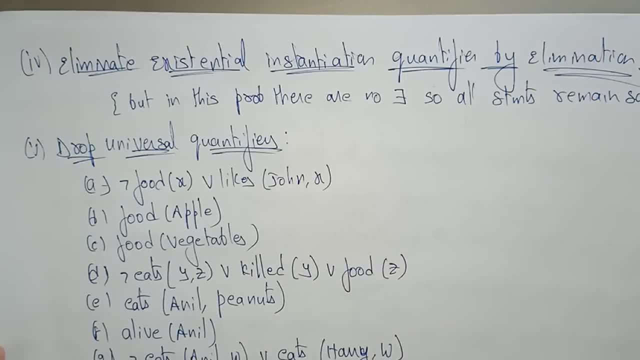 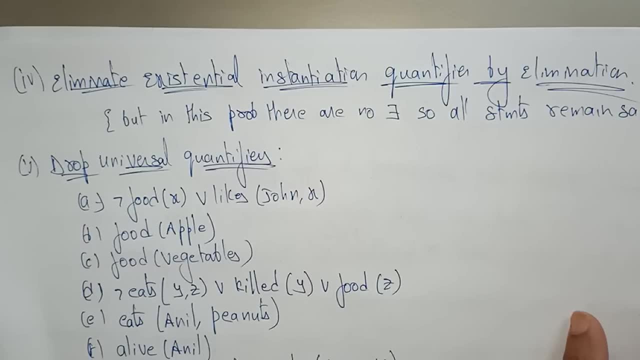 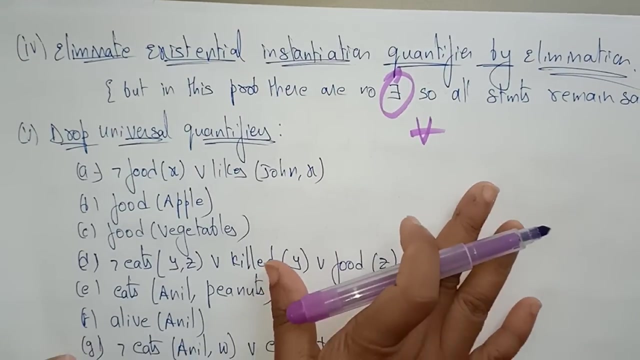 OK, So to avoid the confusion. and the fourth one is: eliminate existential instantiation or quantifier. quantifier by elimination. But here, in our problem, there is no existential quantifiers, because we all use the universal quantifiers only. So here, whatever the steps that are, there they are, remains as it is. 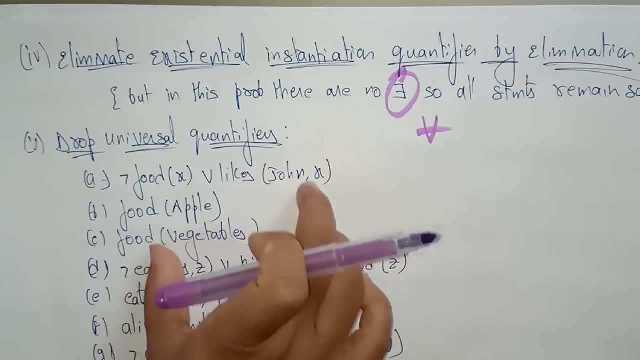 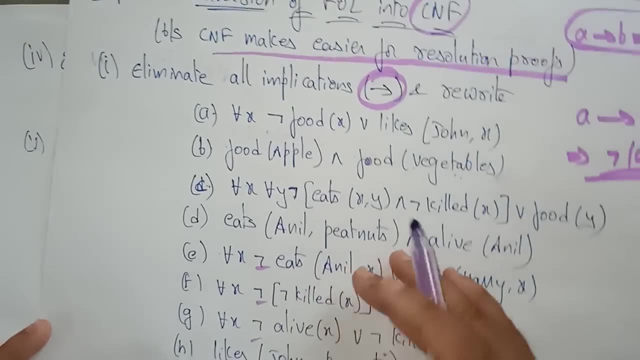 Now drop the universal quantifiers. Now, whatever the universal quantifiers are there, I want to drop it. So there is no change will come if you drop the universal quantifier. So you just drop all the universal quantifiers, whatever it is appeared in the problem. 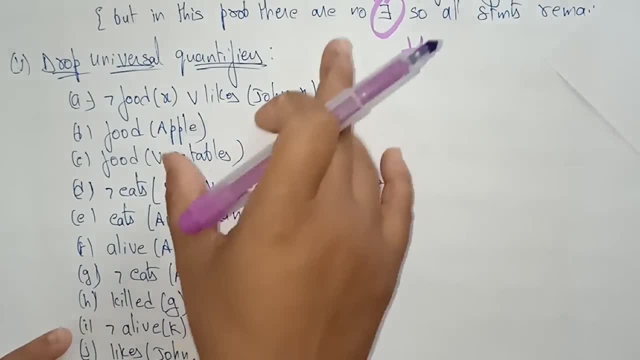 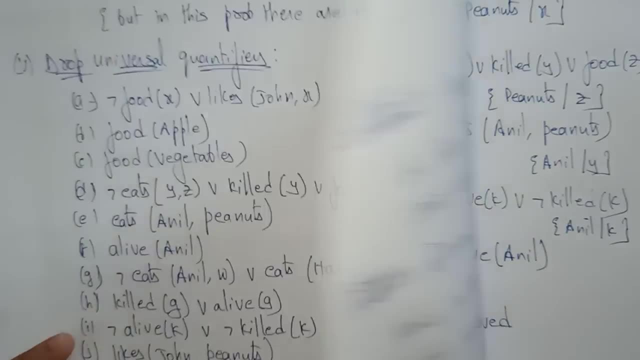 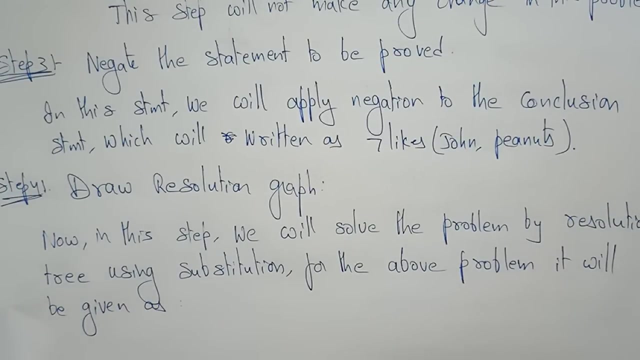 OK And rewrite the statements like this: Just write: just remove the universal quantifiers and write OK. So after dropping that I have to distribute the conjunction. But here there will not be anything, Only change. So these are the steps for converting only for the FOL into conjunctive normal form. 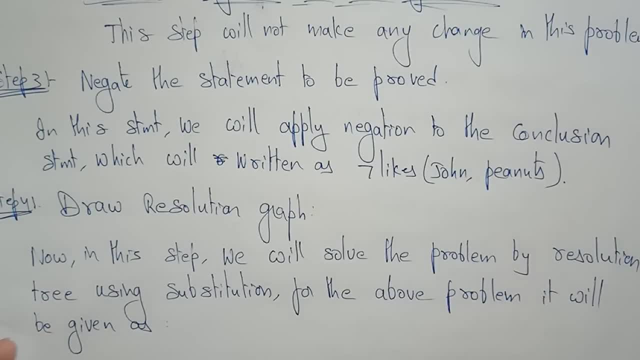 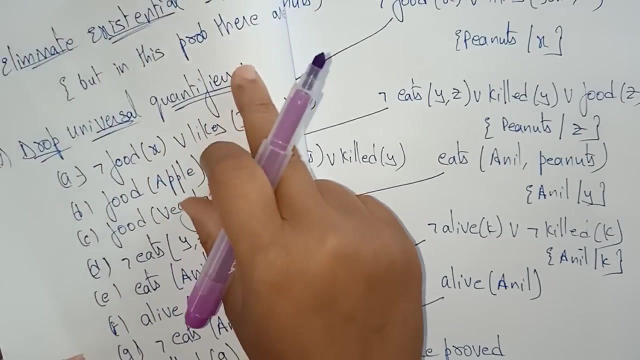 So what I had done, I eliminated the implications. So after that, what I have done, after eliminating the implications, I just move the negation inwards and rewrite. After that I rename the variables or standardize the variables. So after that, what I had taken: eliminate the existential quantifiers, if present, and drop the universal quantifiers. 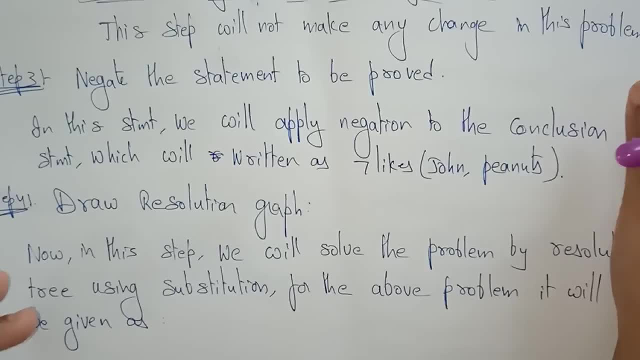 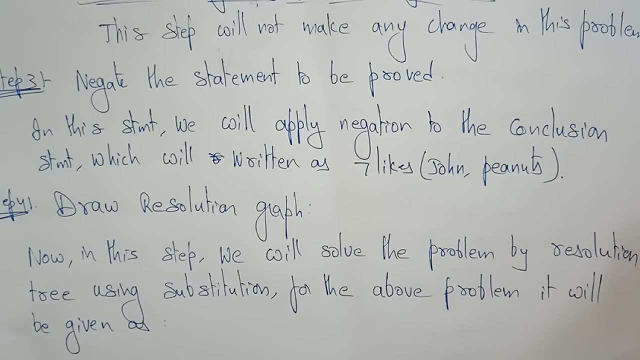 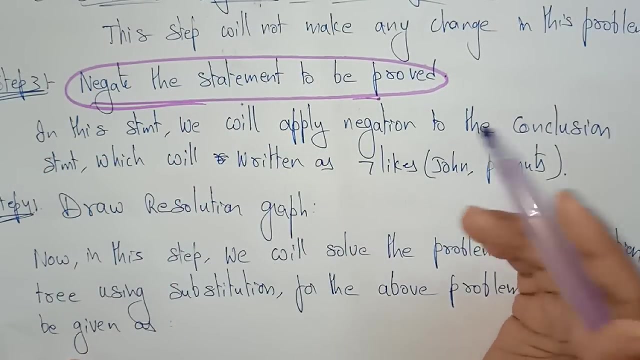 And you'll get some statements Now, step 3. So the step 3, that is, the converting from converting to the resolution steps or step 3.. Then negate the statement to be proved, Whatever the statement that is there that should be negate. 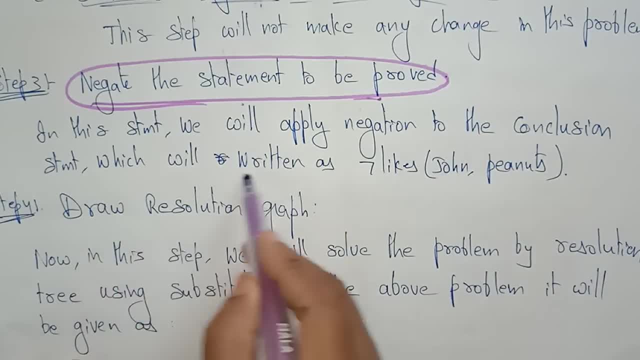 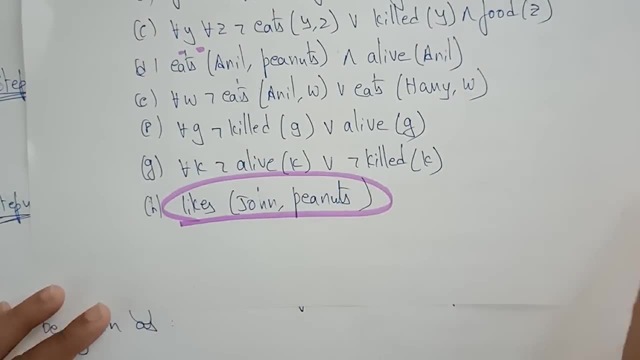 In this statement we will apply the negation to the conclusion statement, which will be written as So here. what will be the conclusion statements? John likes peanut. I'm just taking the negation for that. Okay. Not likes John peanut means John's does not like peanuts. 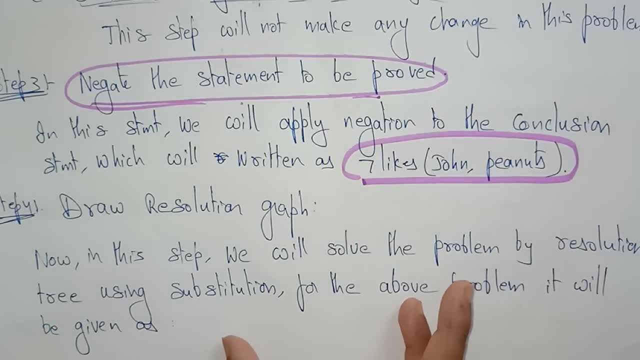 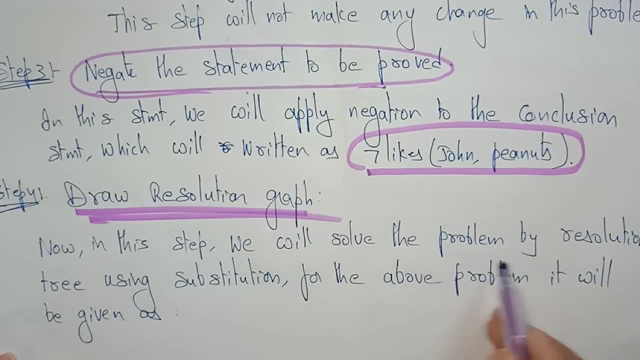 I'm taking this contradiction and I want to prove now the fourth step of the resolution. What is the fourth step? draw a resolution graph Now. in this step, we will solve the problem by resolution tree, using the substitution means, with the help of the unification. 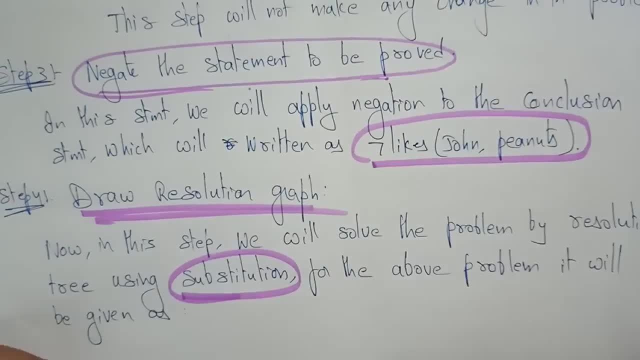 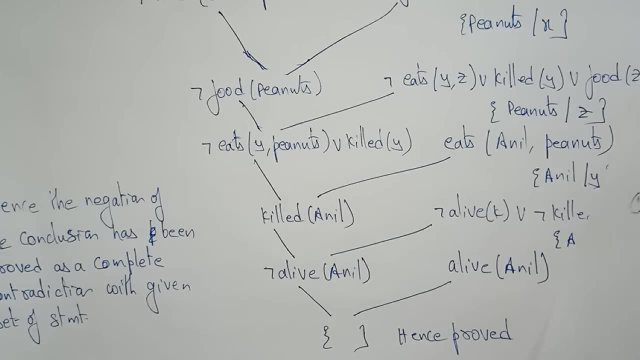 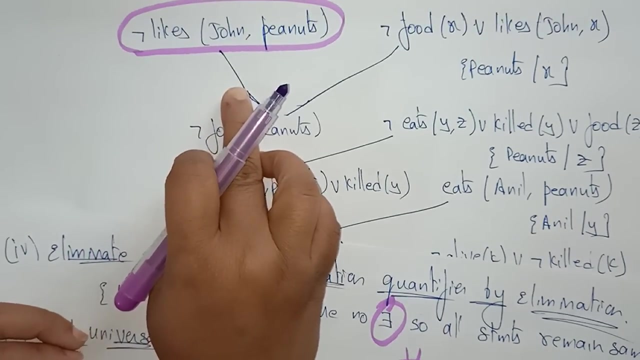 You are going to draw the resolution graph. Let's see how I have. I'm drawing this resolution graph. See here. Okay, So first let me take this, also the first. I am taking the contradiction: John does not like. John does not like peanuts. 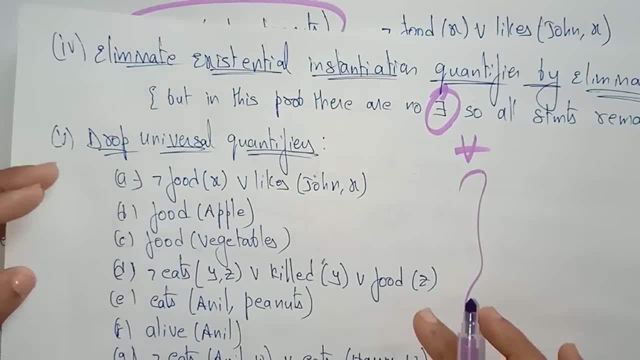 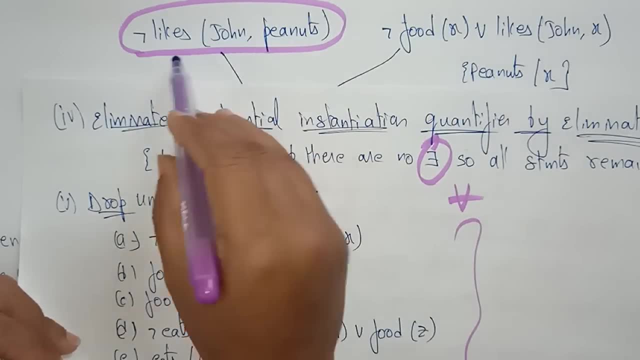 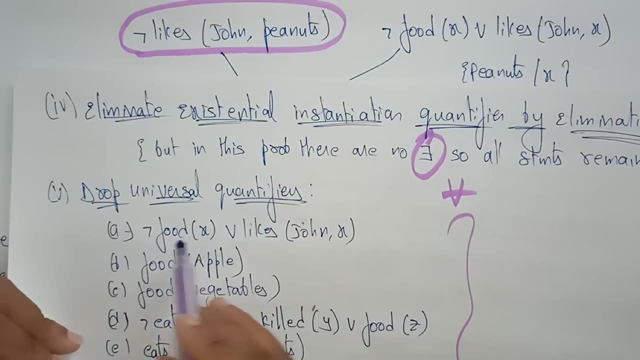 So I need to observe. So these are all the quantifiers. whatever I get in this, I need to be observed. where negation is there? where the negation is there John likes- sorry, John does not like- the peanut. Okay, So here, see in the first statement. 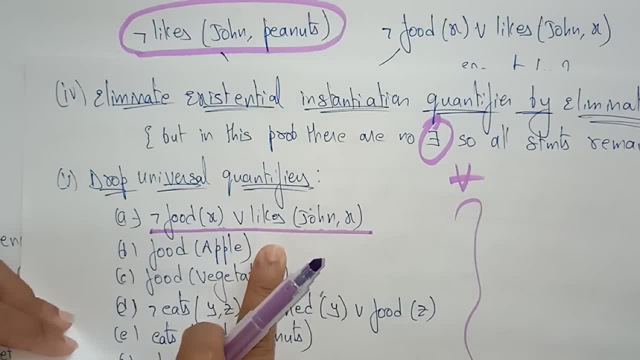 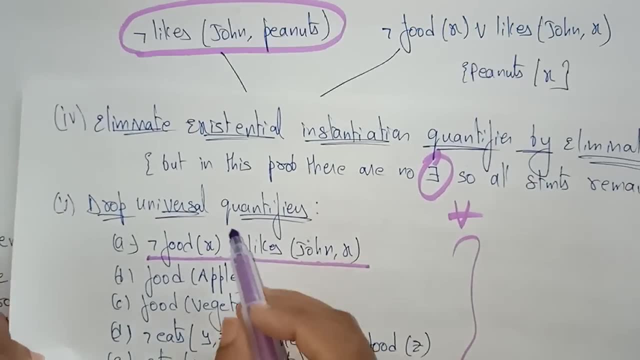 Likes is there, So negate likes. and here the likes is there, So wherever the contradiction statement is there, that statement you need to be checked. So in all these, the contradiction statement observed in the first step itself. So just take that first step. This is the first step. 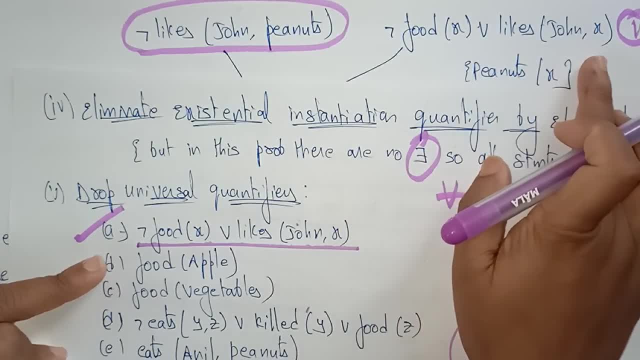 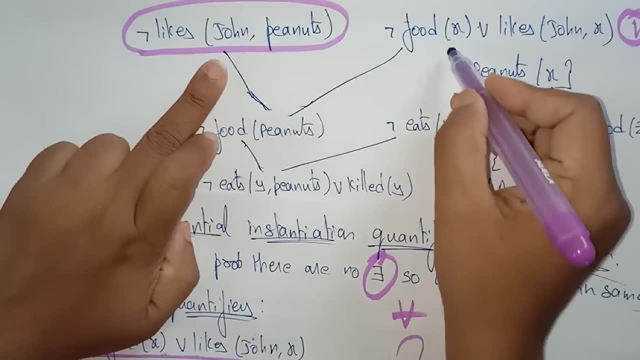 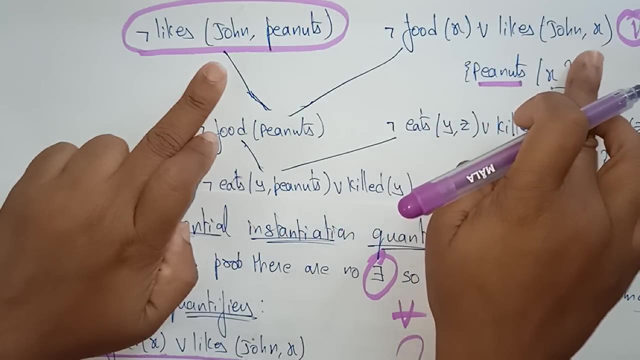 I'm taking negate food of X or likes John, comma X. So now, here in this I'm going to use a unification method: substitute in place of X, substitute the peanuts. So now I it becomes negate, I get food of peanuts or, likes John, come up peanuts. 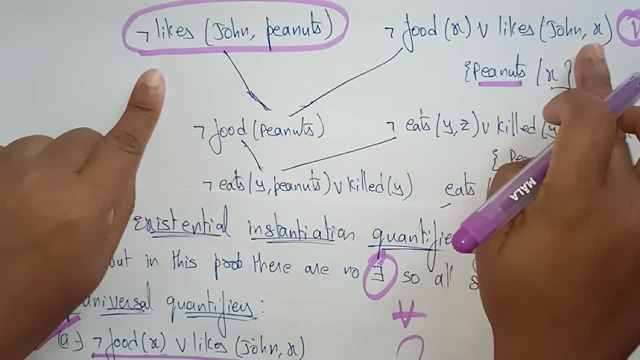 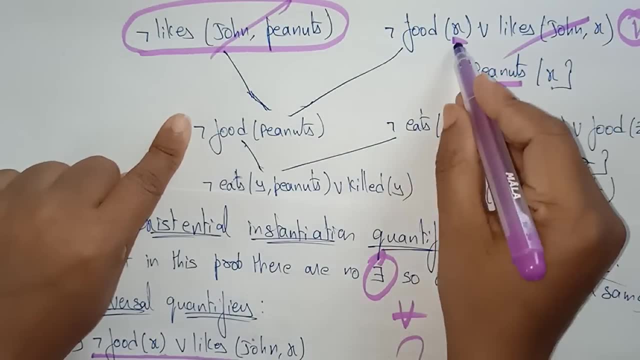 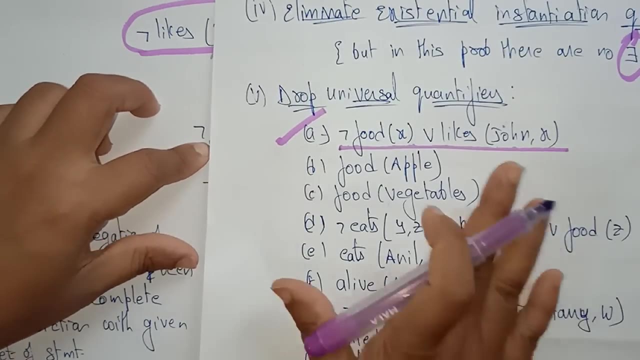 So here: likes John come up peanuts and not likes John come up in it. So these two will be cancelled and in place of X, the peanuts will be replaced. So this I got: negate food: come up peanuts. Now in this quantifiers, drop Universal the final statements. wherever the contradiction of this food will, that has to be taken. 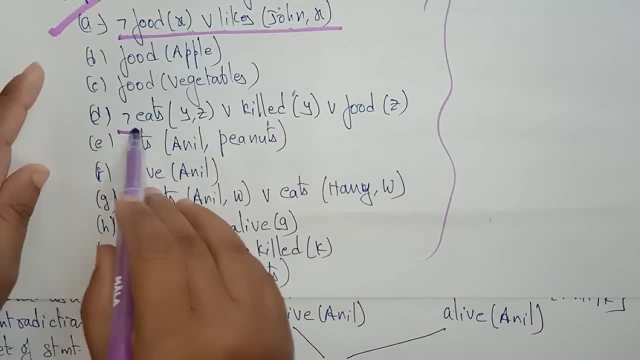 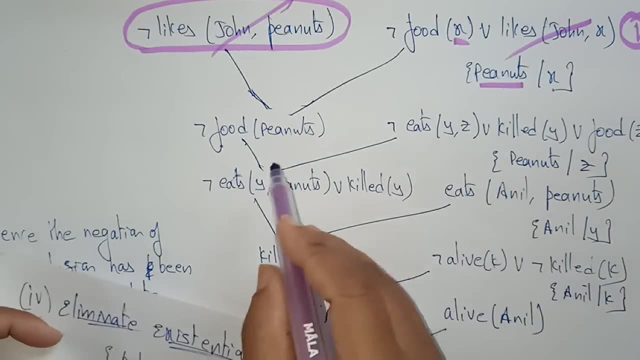 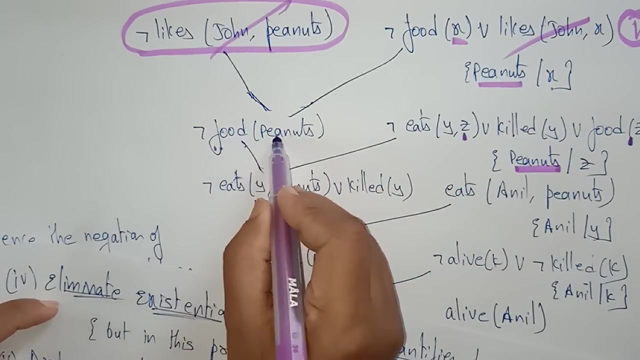 So where is the contradiction here? Contradiction here is in this statement: Food. Okay, so just write this food, this statement here. Now, in place of Z apply the peanuts, in place of Z apply the peanuts. So here the negate food, come up peanuts, and this is simply food. come up food of peanuts. 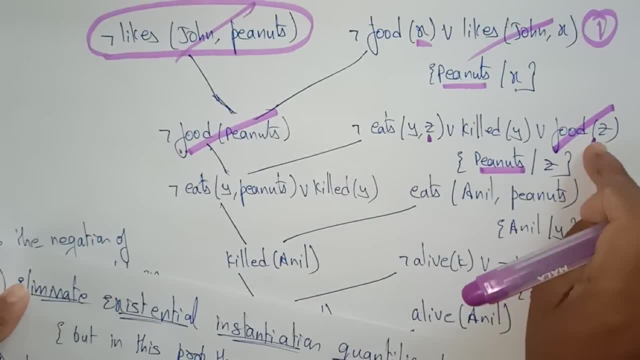 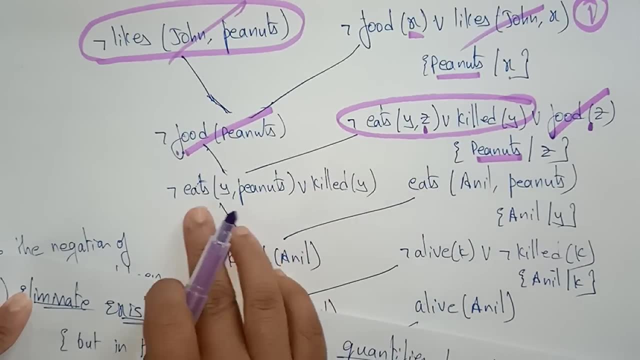 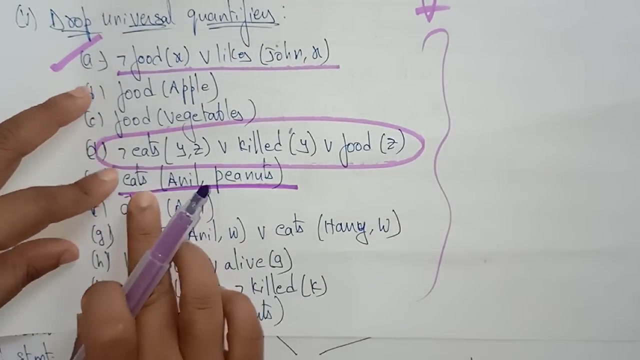 Negate food of peanuts and food of peanuts will be cancelled. in place of Z, I substituted peanut. Now only these statement is remaining: So bring here. So now check the negate eats wherever the eats is there that you have to be taken. So here, in this case, the eats is there, here the negate eats and here simply eats. is there? contradiction statement. 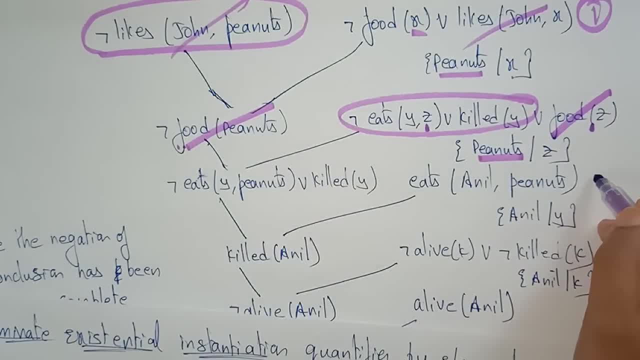 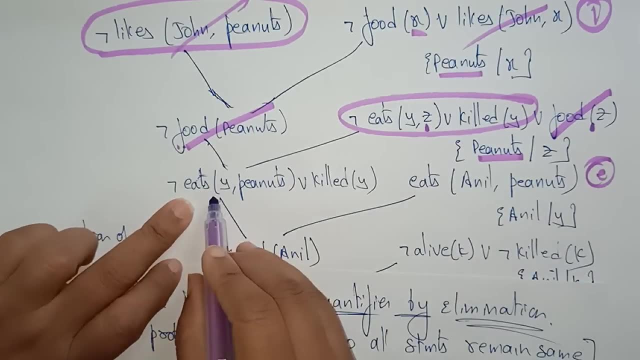 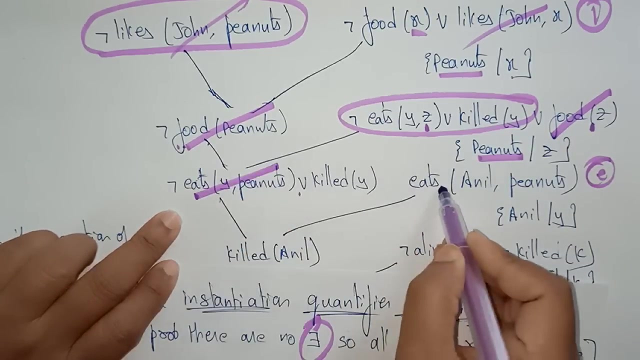 You need to be take. so I taken that statement E. Okay, so in place of Y I'm substituting Anil. So negate: eats Anil, come up peanuts or killed wife. So this is negate Anil come up peanuts and this is simply Anil, come up peanuts.